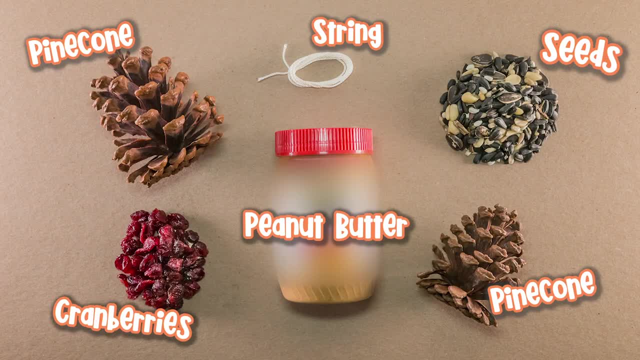 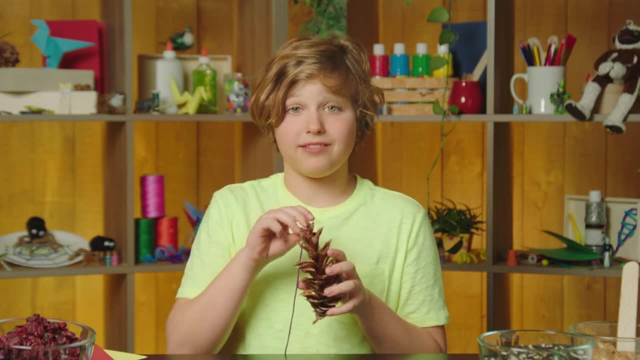 peanut butter, seeds, string and dried fruit like cranberries. For step one, we'll need our string and our pine cone. You can use any size pine cone you want And you can make so many of these. Tie it right to the top end of the pine cone. 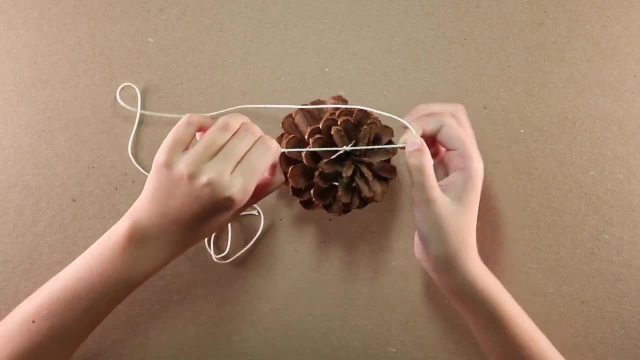 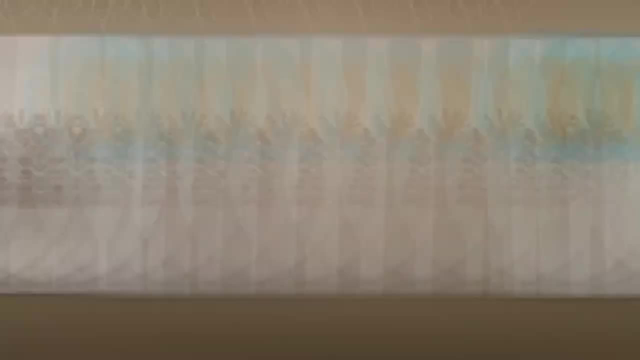 and make sure it's good and tight. This is so we can hang it up once we're done. Now time for the fun part. Let's smear the peanut butter all over the pine cone. Let's get lots of yummy peanut butter into all the gaps and little edges of the pine cone. 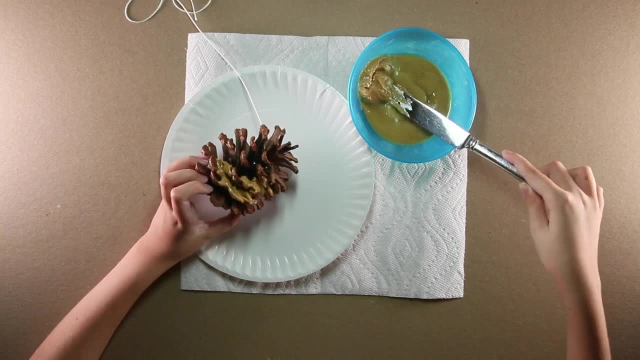 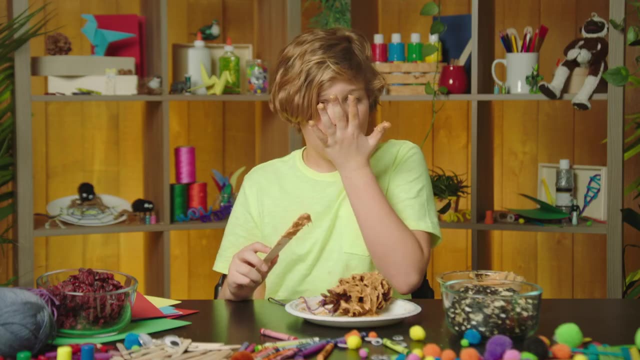 You can use crunchy, sticky peanut butter or smooth peanut butter. That's up to you. This is where things can get a little messy. It's a good snack for birds and for me. All right, I've got my pine cone all covered. 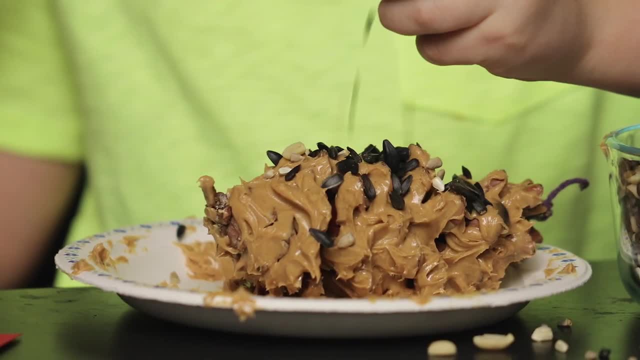 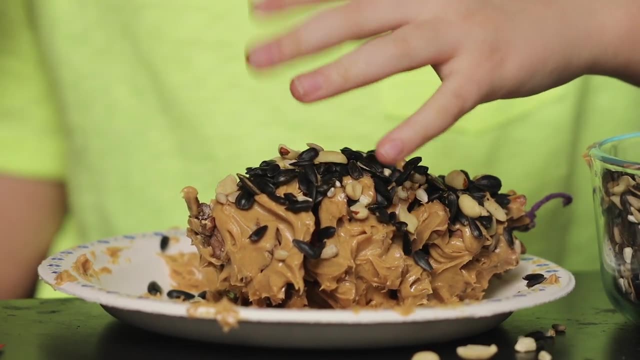 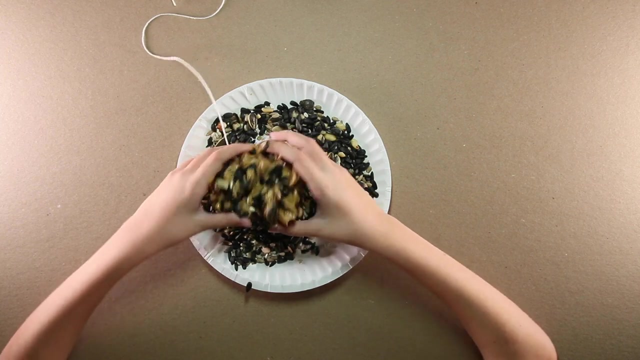 in that sticky peanut butter. Now let's put our seeds on. Save some peanut butter room for the cranberries, but go all out. Roll your peanut butter pine cone around in the pine cone. We want to make sure it's completely covered, so there's plenty for those birds to pick off and snack on. 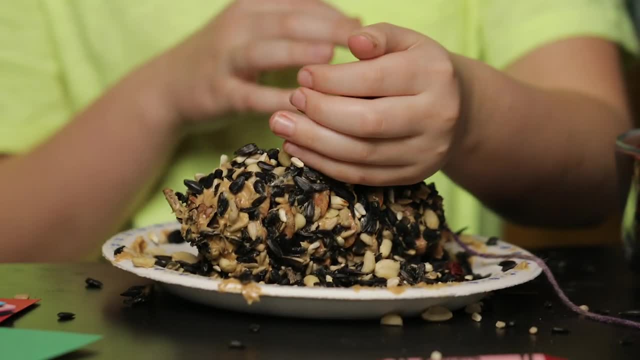 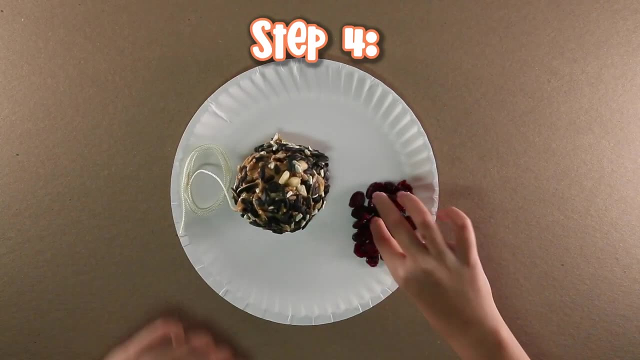 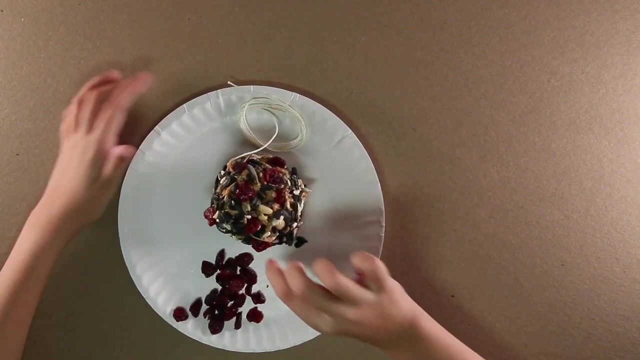 For the finishing touch, cranberries, Dried fruits, go really well with seeds and peanut butter. if you're a bird, You might have to squeeze the cranberries in, because the seeds kind of covered up all the peanut butter spots. Do you guys like fruit? 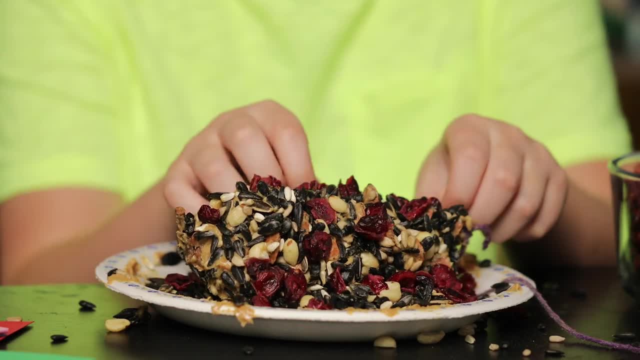 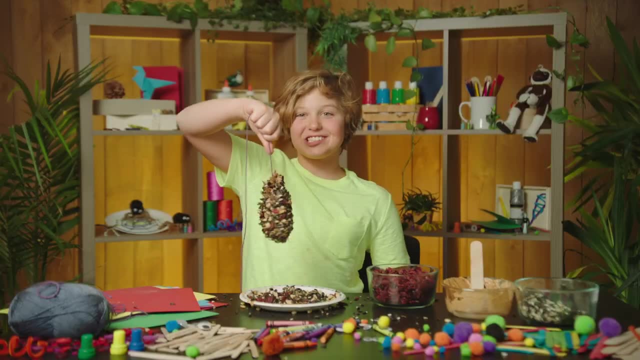 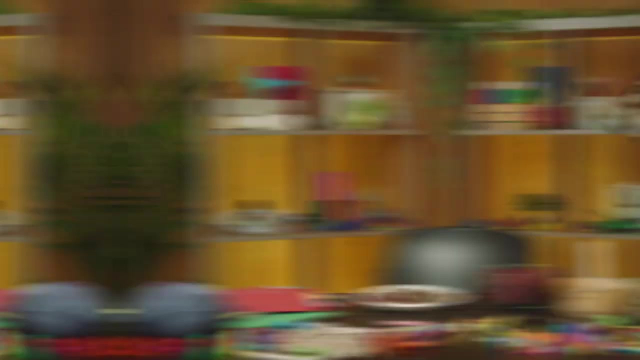 I do. I don't like cranberries. I don't like cranberries, though. I like mango. I like cantaloupe. I think that's pretty good. All finished, This looks delicious, doesn't it Time to go get it to the birds?